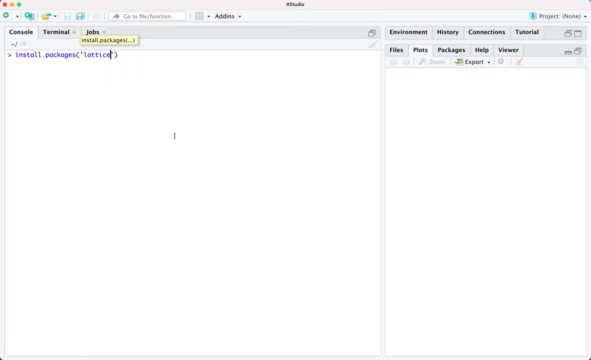 install packages and then the name of package. so the name of package is the lattice. now, in my case, I have already installed this package. now, once your installation is done, we have to load this package, so you need to write library and then name of the package. now for visualization, we need a data set and 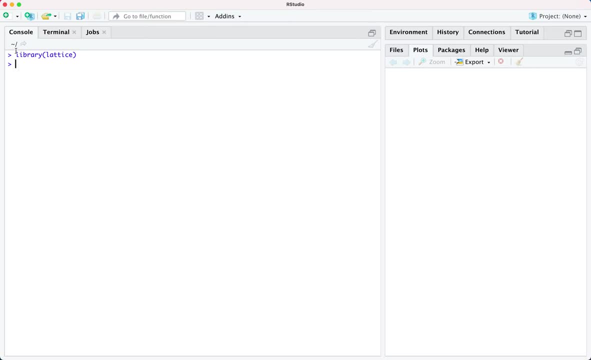 for this exercise I'm going to use a data set already available in our environment, so for that you need to load this package data sets. now, this package actually comes with multiple data sets and one of the data set name is empty cars, so this is the data set about cars. so, as you can see, so 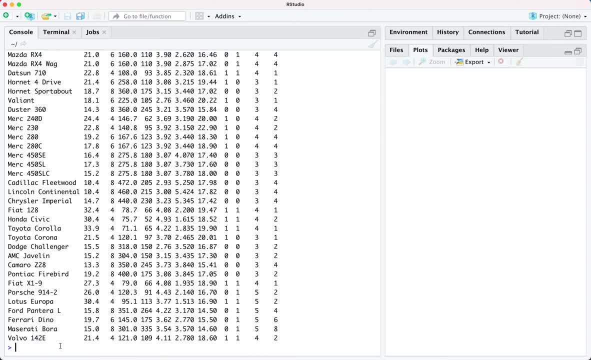 the name of the data set is empty cars, so I want to see how many attributes are there so I can simply write str. okay, so we have a few attributes and, as you can see, we have here. we have a few attributes and, as you can see, we have a few. 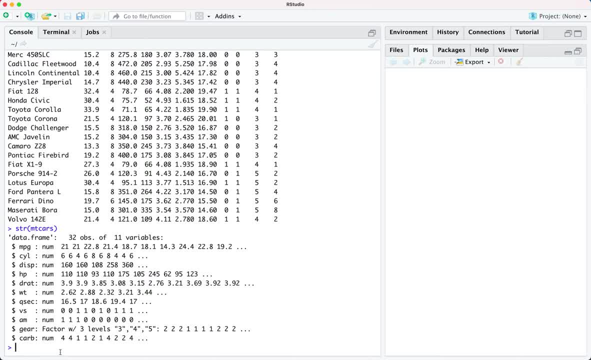 uh, all of them are numeric and one of the attribute, uh, it's showing factor. so in your case it will show it as numeric, because i have changed, uh, this attribute type to factor. so just to understand what's the factor mean. so when you have a categorical type of attribute, that attribute 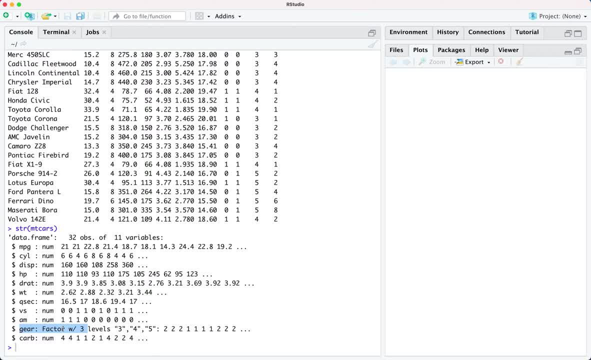 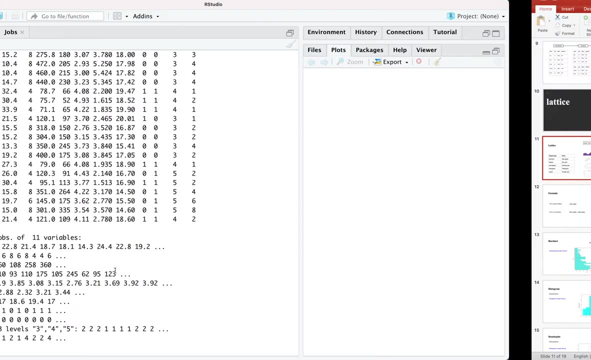 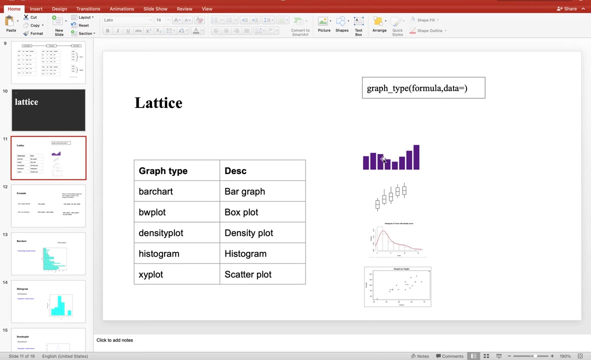 is either stored as string or numeric, so you have to explicitly state that this attribute is a factor attribute. now, uh, we have this data set. now we will talk about the graphs we are going to generate. so we are going to generate these five types of graphs: bar chart, as you can see here. 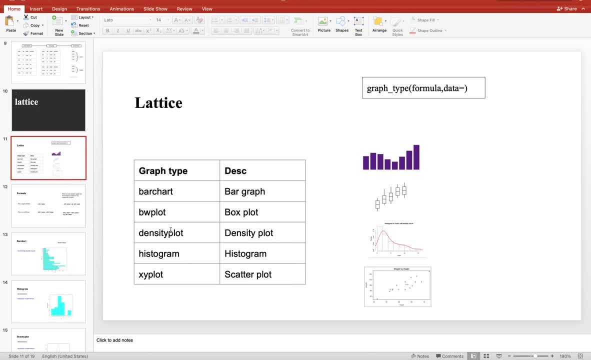 box plot, density plot, histogram and scatter plot. so in lattice package uh formula to generate any graph looks like this one. so first you specify type of graph. so here is the, here are the types of graph. and then you specify the formula, and then you specify your data variable, the data or the object. name of object having reference to your 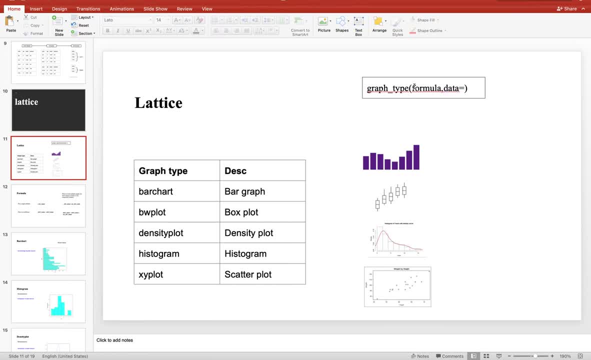 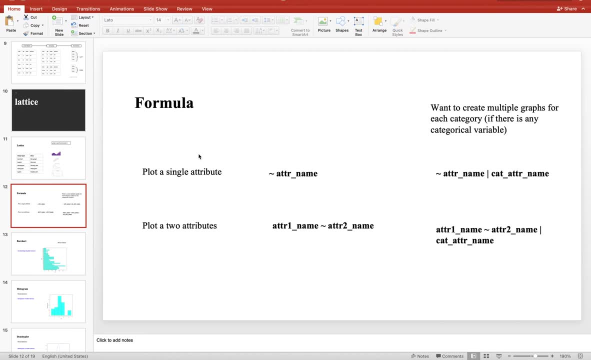 data set. so, uh, here the question is uh. so here the question is uh, is this formula like how we are going to write this formula? so for that i have prepared the slide and i will take the simplest example first. so let's say we have a single attribute we want. 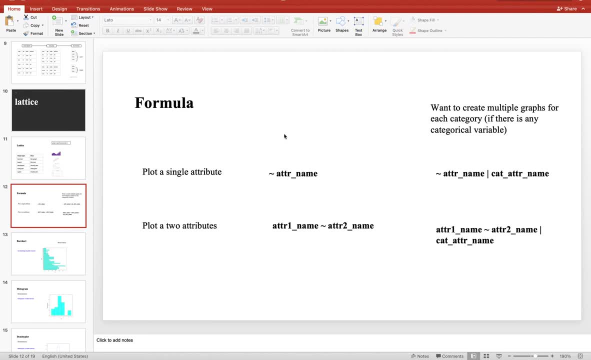 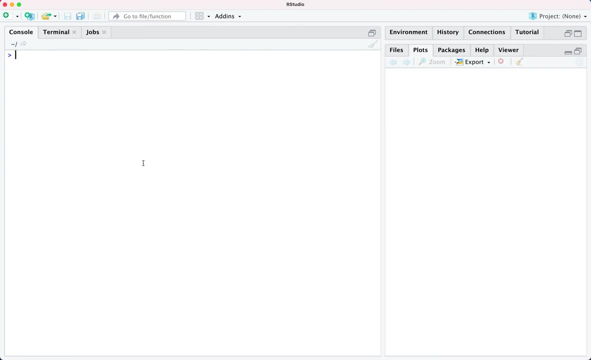 to plot a single attribute. in that case, your formula will include the name of the attribute and it will start with a tilt sign. okay, so we will go to back to the r studio. let me clear the console. so here, uh, just to have the name of attribute. so let's say, uh, here i want to plot. 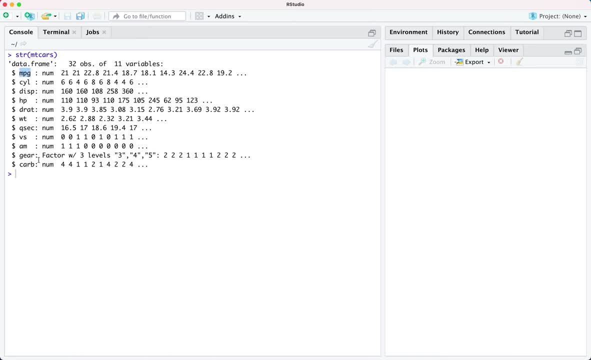 this attribute, the name of that attribute is mpg and i want to plot a histogram. so from the slide we know, in order to generate any graph- uh, the command look like you have to specify the graph type. so the type of graph is histogram, then you have to specify 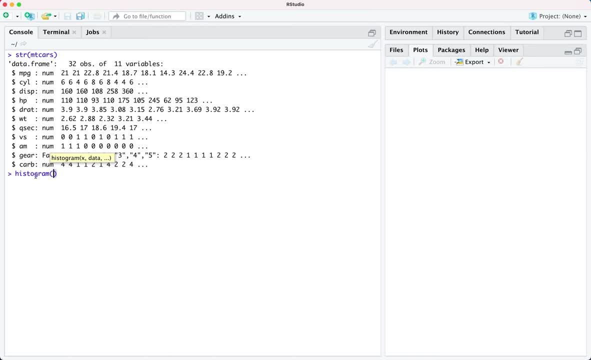 the formula. so in this case we have a single attribute. so we will write the formula- tilt, sign and the name of the attribute, and then you have to specify where is your data stored. so empty cars is the name of the object or name of the variable having your data. 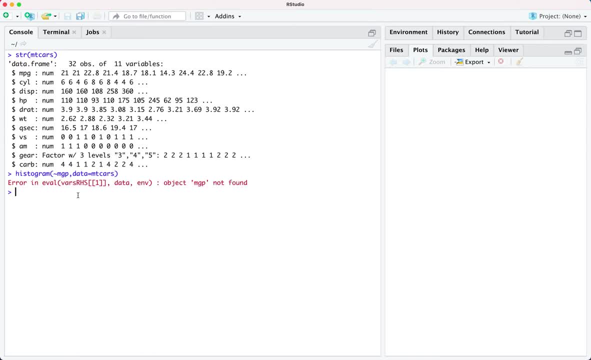 so you write here empty cars. so, as you can see here, we got a error. so that's a good thing. error is: i have wrongly specified the name of variable, so let me correct it so as you can see here: uh, we have a nicely plotted histogram and you can do similar with other plot as well. so if you want to generate a box plot, 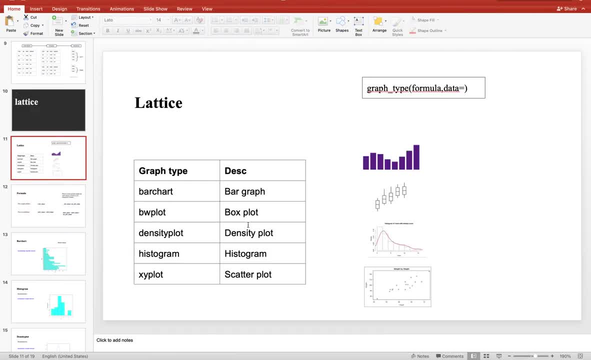 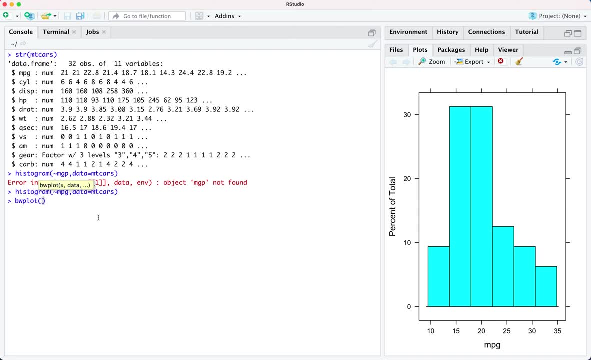 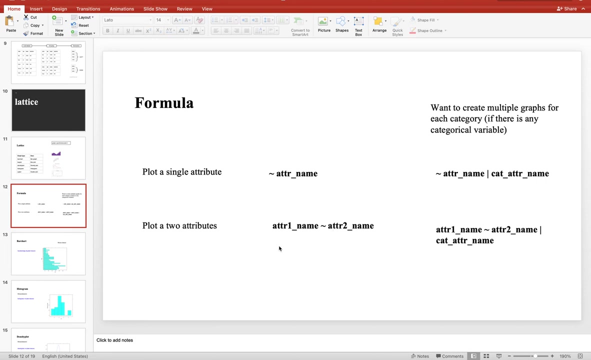 so if we go back here for box plot, then graph type is bw plot. so you write bw plot, tilde sign, mpg data, empty cars. so you have a box plot. so similarly, uh, you can use other graphs. now, uh, i'm going to use graph with two attributes. so when you have two attributes and when you want to generate a scatter plot, 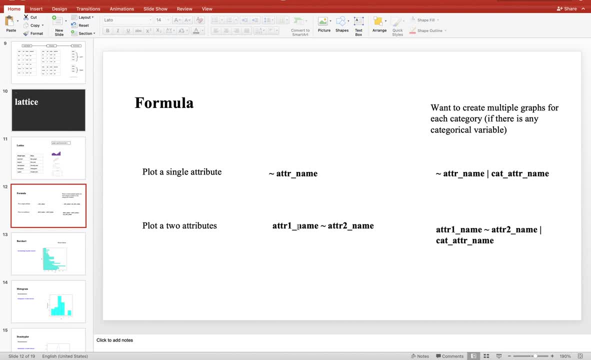 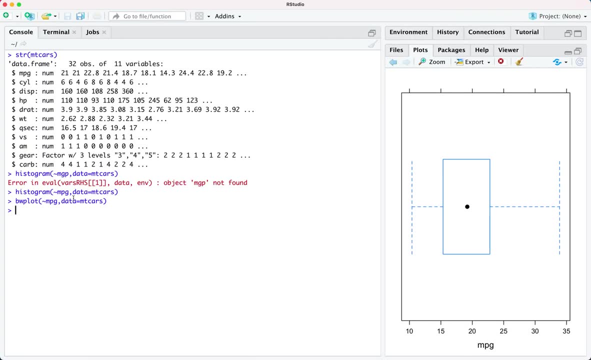 uh, the formula will look like this. so first you have to specify the attribute name: first attribute, first name and then the second attribute name. so here let's say, i want to plot a scatter plot between attribute mpg and let's say wt, what? so i will write the graph type for a scatter plot. 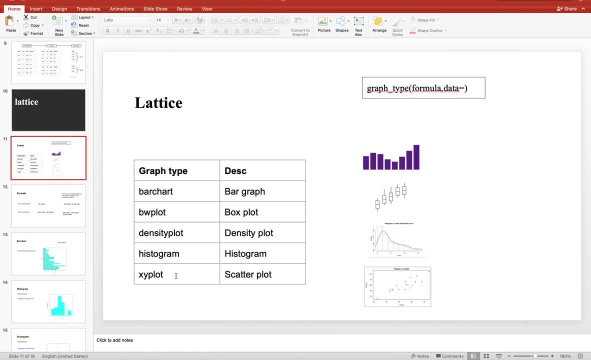 and if we go back to the bottom here you can see that it's a scatter plot. so this is a scatter plot, uh, data that i first added. so we now want to write the graph type for scatter plot and if we go back to our slide, the scatter plot graph type is x- y plot. so i will write x- y plot. then i have to specify: 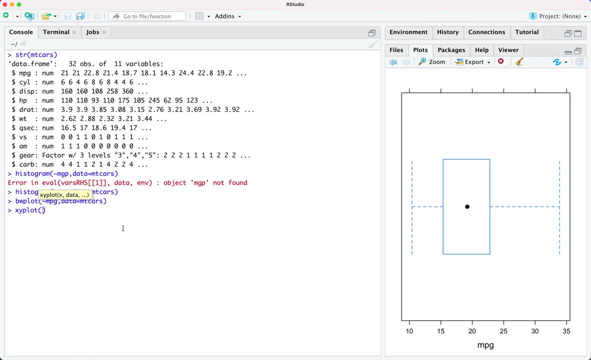 the formula. so in this case i'm having two attributes. i will specify wt, tilde, mpg, and then i will specify mt- cars. so, as you can see, it has plotted a scatter plot and this kind of plot can help you to understand the relationship between two attributes or variables. so 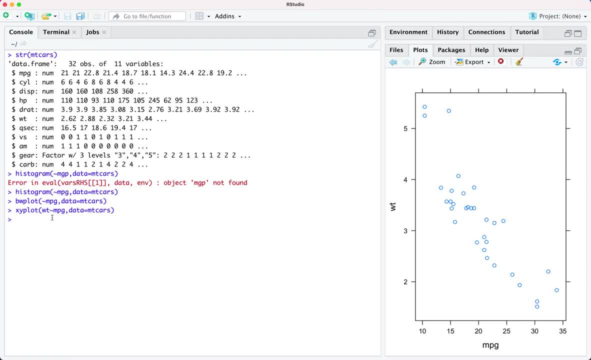 just to revise. so if you want to plot a single attribute, your simplest. this is the your simplest formula: the name of the attribute started with a tilde sign. when you have multiple, when you want to plot multiple attributes- so like scatter, plot involve use of two attributes. in that case you. 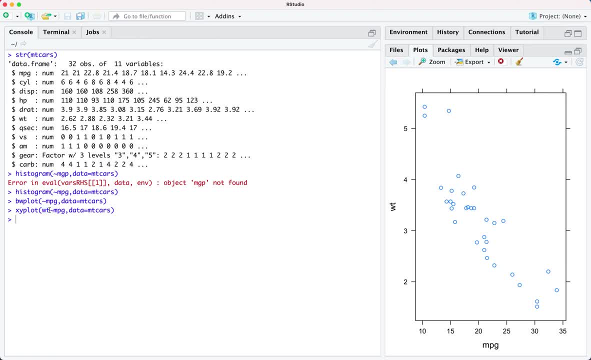 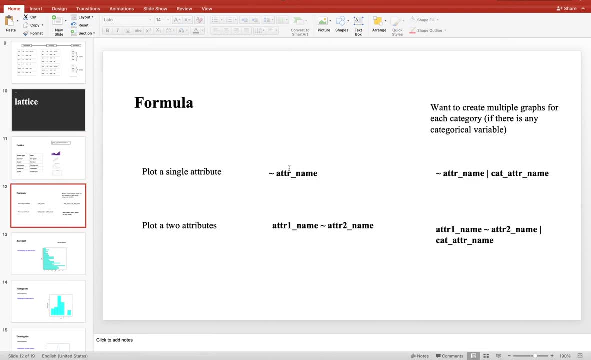 specify both the attributes and between them you specify tilde sign. now, uh, what is the meaning of rest of the formulas? now, sometimes we have some categorical type of attributes in our data set, let's say gender in a salary data set, and we want to understand, uh, the salary, uh. 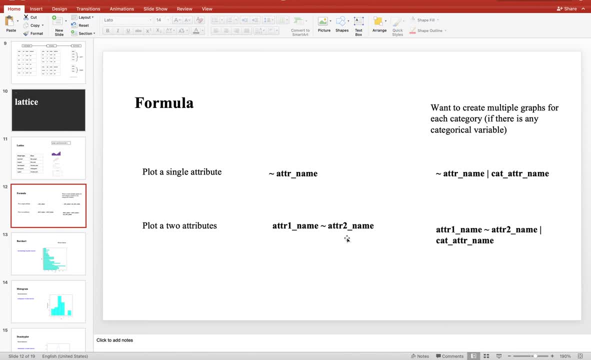 among so salary on the basis of gender? gender like, is there any bias in the salary? so you want to generate multiple graphs for each gender. similarly, if you have a, let's say, employee salary data set and you also have a educational level and you want to see, you want to generate a graph for each educational level in terms of salaries. so 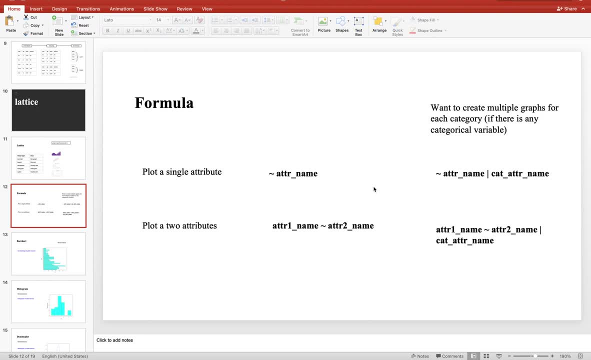 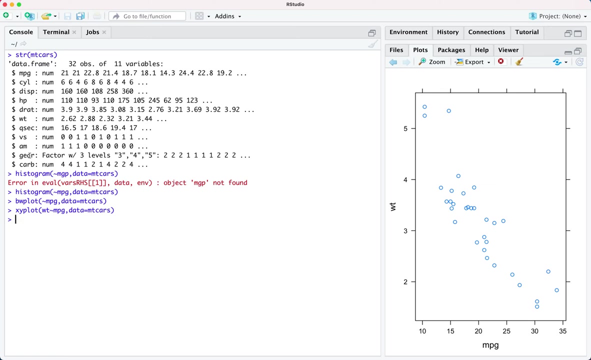 how we can do that. so, using lattice, it is very simple. you will use your formula and you simply use this syntax, so you write this one and then the name of your categorical attribute. so here, uh, let's say uh, i i want to generate uh two, uh box plot for uh, this attribute, and so not to uh box plot for. 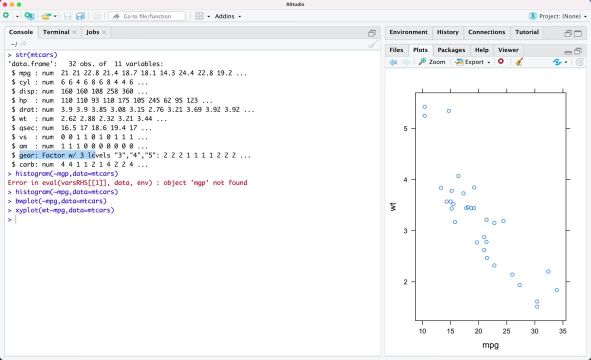 mpg for each factor of gear. so, as you can see here, uh, this attribute has only three different values: three, four and five. so i want to generate a graph for each of these value. so how i'm going to do that? uh, select whatever graph type you want to plot. so i will select bw plot. i will write mpg. 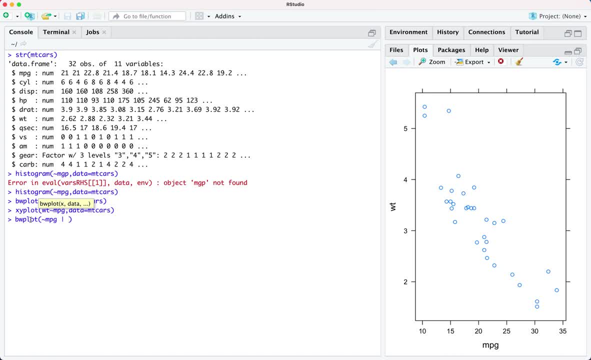 and then i will specify the categorical attribute: name data: empty cars. so it will uh select mpg data, let's say where the gear value is three, and then plot that data. then it will select all the mpg data where the gear values for, plot that data and so on. so when i hit enter i can immediately see three. 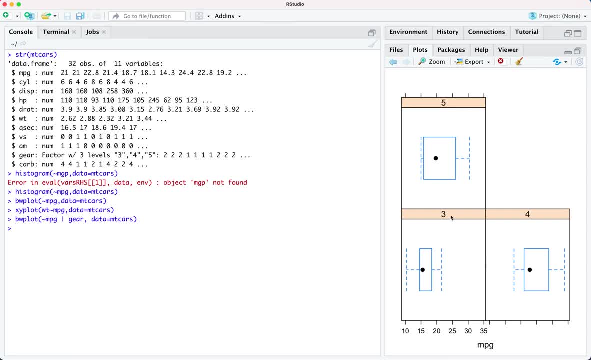 graphs. so this first graph is for gear value three, this second graph is gear value four and this is the third graph for gear value of five. so you can see, uh, it's very easy uh to generate graph for each of your factor. uh, now let's do the same with our xy plot. 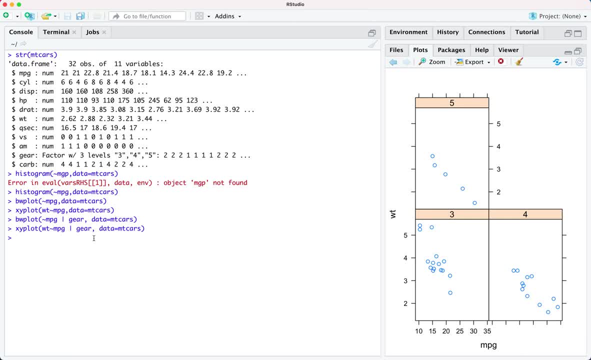 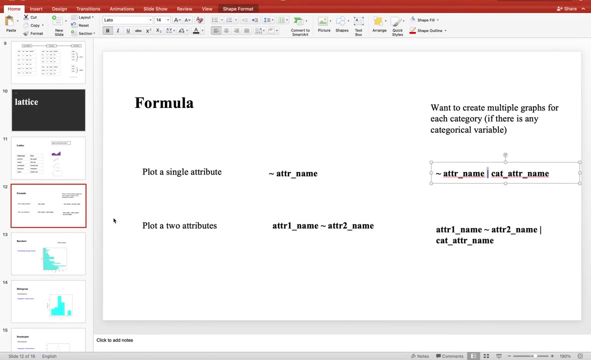 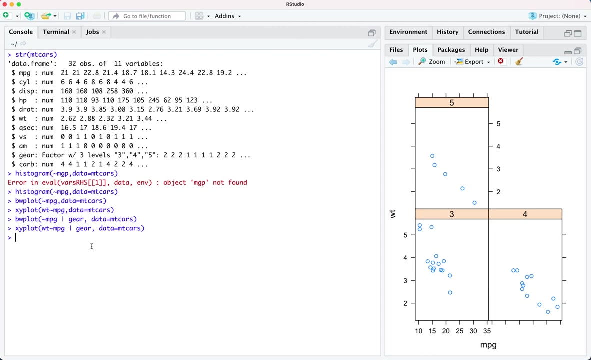 so for each of the factor level you can see, uh, the relationship between mpg and wt attribute. so we have a plotted histogram, box plot, scatter, plot. so let's plot density, and bar chart, bar graph, so bar chart. let's say i'm like, say I'm going to plot this for mpg. so what I have done, I have specified the. 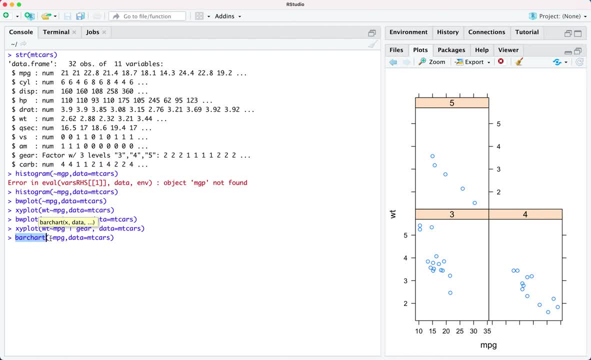 graph type. so this is the type of graph I want to generate. then I have specified the formula. so formula is very easy to remember. if you have a single attribute, it will start from tilt. if you have multiple day two attributes, you put the tilt in between and then you specify the name of your variable or object holding. 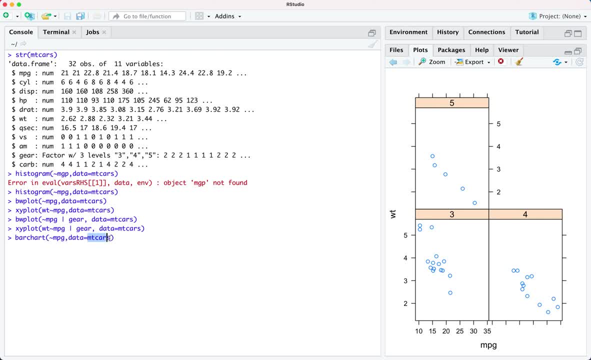 your data set. so D. so our data set is stored in a variable- empty cars. so I have specified data equal to empty cars. so here it looks a bit weird. let me you do this with two attributes now, so, as you can see, you can use bar chart with. 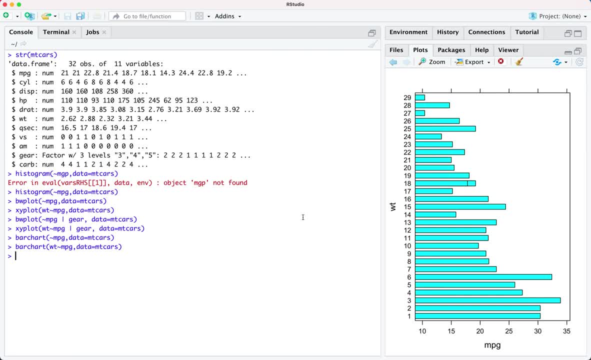 one variable as well, but you cannot make much sense out of that. but when we use two attributes, it became quite clear to us. so, so this y-axis is showing WT and X, X the axis showing mpg. so for each of the WT value we have the corresponding mpg. 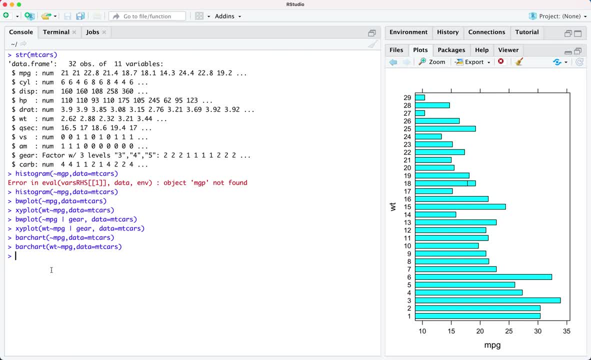 now I'm going to also show you how to generate density plot, so this plot can help you understand the solution in your data. and for that I'm going to use, let's say, this attribute, HP, and I'm going to use this one, so this one will be our. 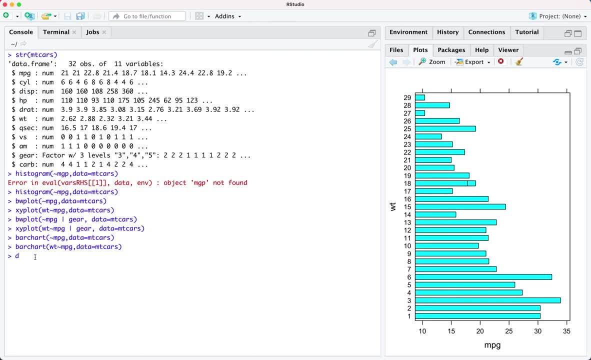 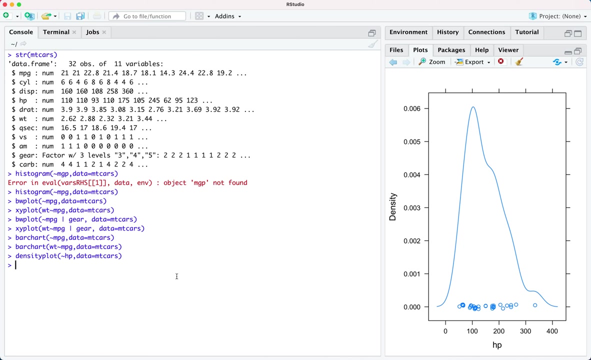 so you have to specify the graph type. so in this case, density plot formula. so we are going to generate a graph for hp distribution. so hp data: empty cars. so this is the density plot for hp attributes. so i hope you understood some of the thing out of this tutorial. just to revise thing. 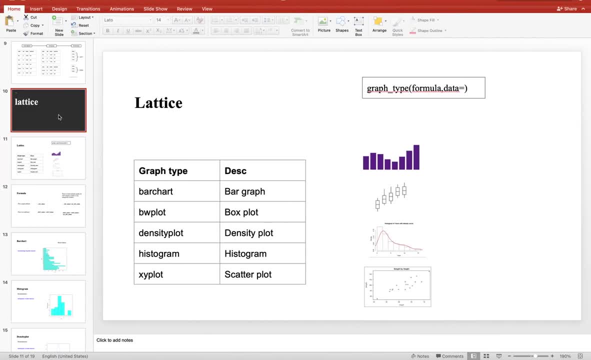 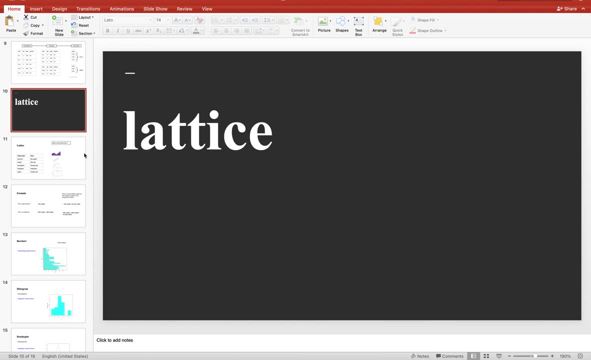 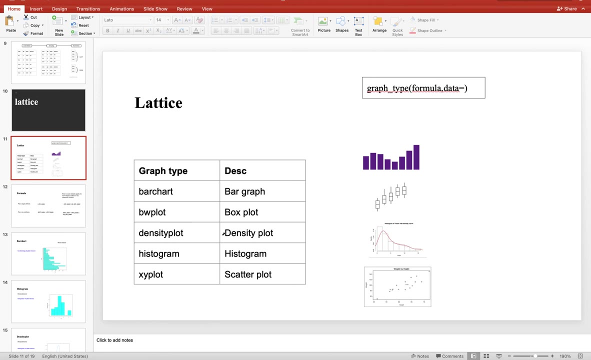 again. so we have seen in this tutorial how to generate data visualization using r. so we have used this very nice package, lattice, and in this, using this package, we have seen how to generate bar chart, box plot, density plot, histogram, scatter plot and so on. so we have seen how to generate